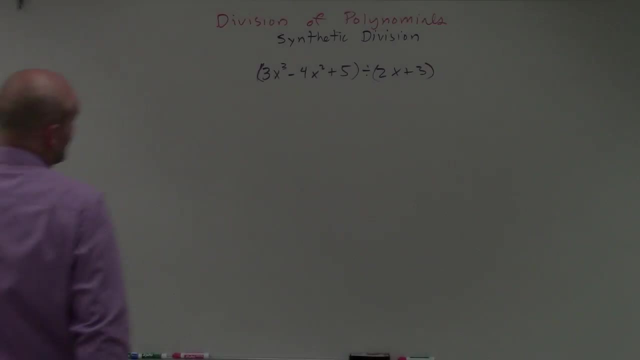 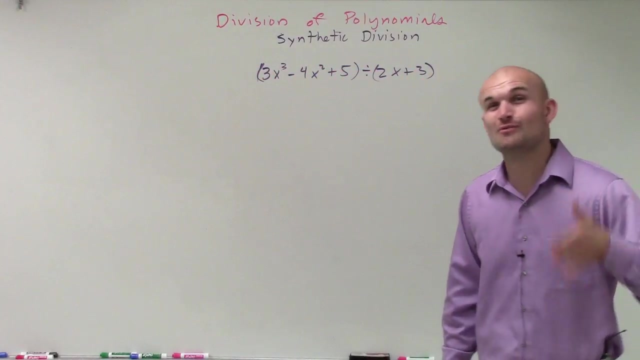 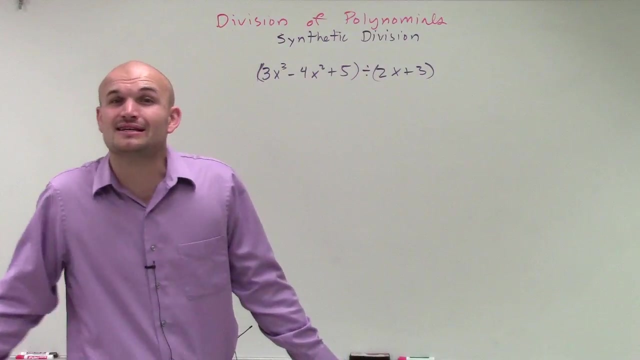 Okay, so here's going to be what we're going to finish it off with, and I put this problem in there because a lot of times we'll do so many problems when we have a binomial in the form of x minus k that students look at this and say, oh, 2x plus 3, well, we can't do synthetic division. 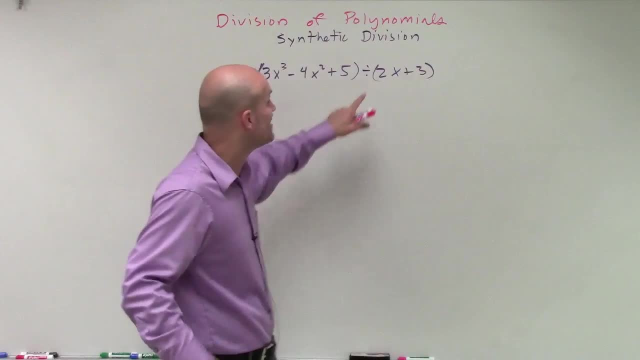 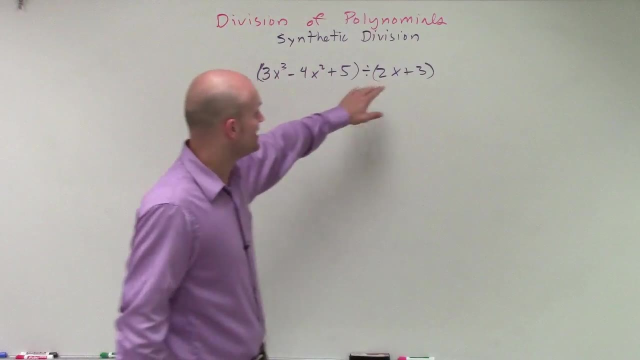 because it's not in the form of x minus k, but it is. We can have a coefficient for x. The only important thing is we need to make sure it's a binomial and also that it's linear. and we see that, yes, this is a binomial, has two terms and my variable x is raised to the first power. So 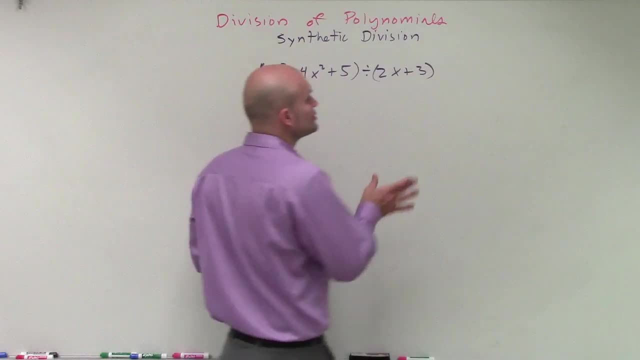 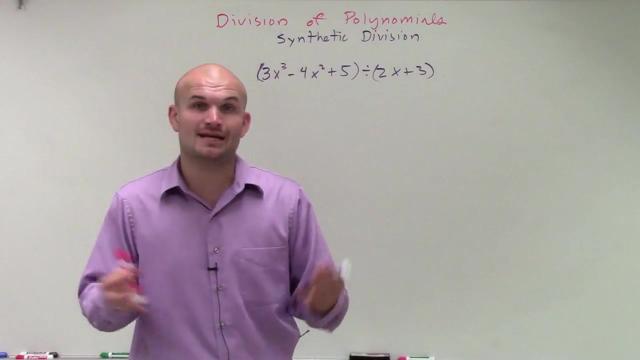 therefore, it satisfies all the requirements. Now, when determining what exactly the value of what we call our k that we're going to look for- remember, on those easier problems- what I did is I set it equal to zero, and we're going to do the exact same thing. So I'll take 2x plus 3 and set 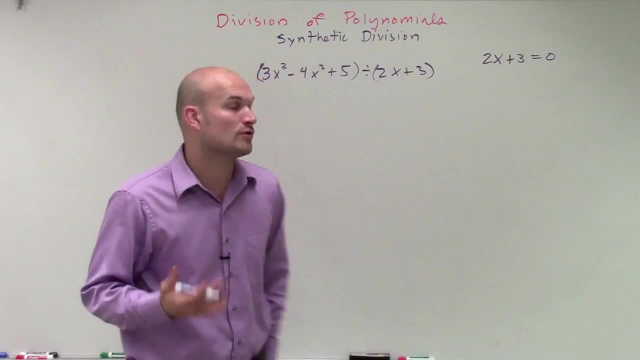 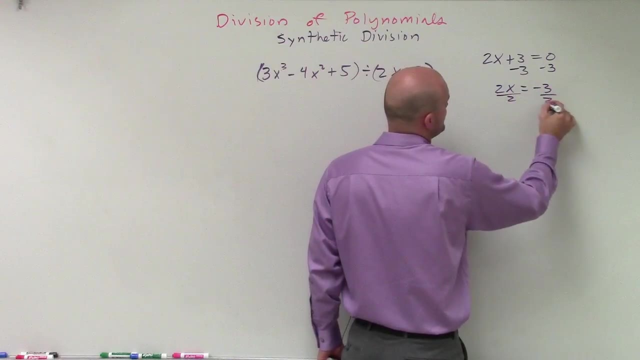 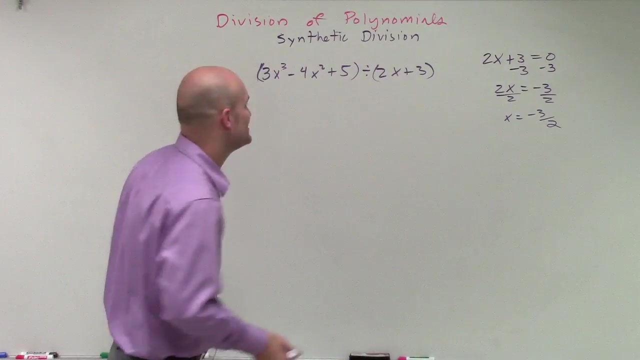 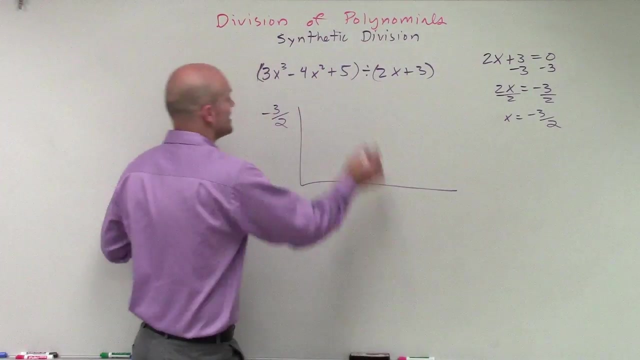 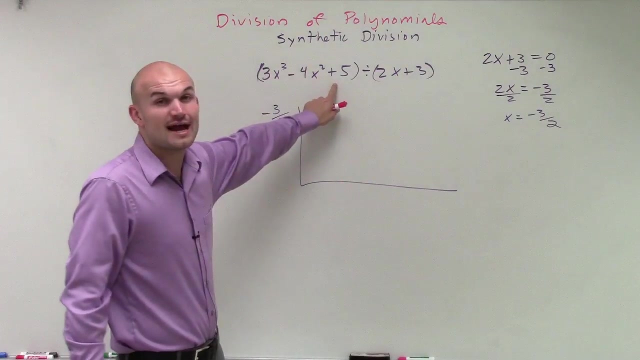 it equal to zero. So what is this value of x that I'm going to use for my synthetic division? Well, we need to solve for x. So I subtract 3, 2x. x equals negative 3, divide by 2, divide by 2, x equals a negative 3 halves. So, yes, we're going to do some fraction work, which is probably not going to be too bad. but let's just go and take a look. So I have a negative 3 halves. put it outside my box and then remember we have to use our coefficients and our constant, but we need to make sure we're going in descending order. In this case, we notice that I have a missing term for my linear, so therefore I need to include a zero as that coefficient. So I have 3,. 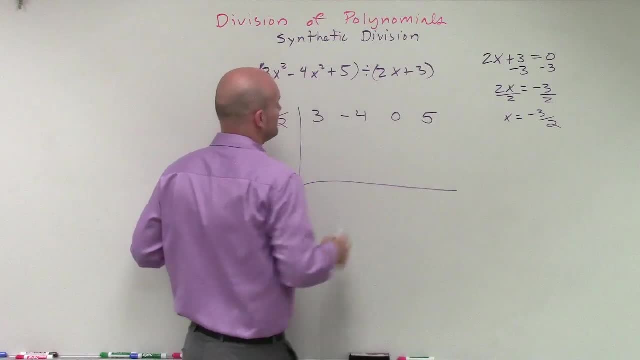 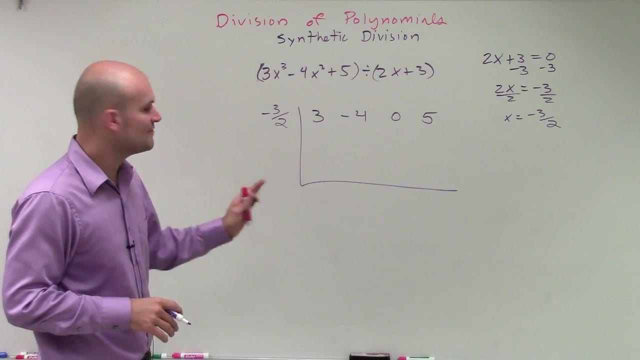 negative: 4,, 0, and 5.. Alright, so then again, remember: what we're going to do is we're going to bring down our first term and then multiply. So I have 3, bring it down just 3.. 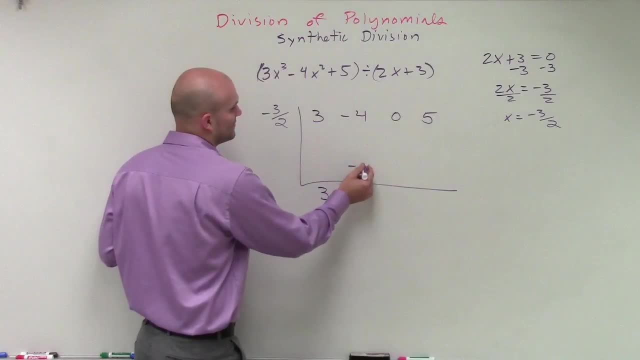 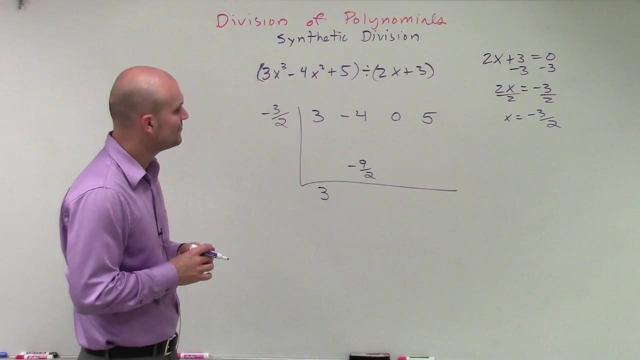 3 times a negative 3 halves is going to be a negative 9 halves. Now we need to make sure we add negative 4, negative 4 plus a negative 9 halves. So the important thing to do to that is to convert it. 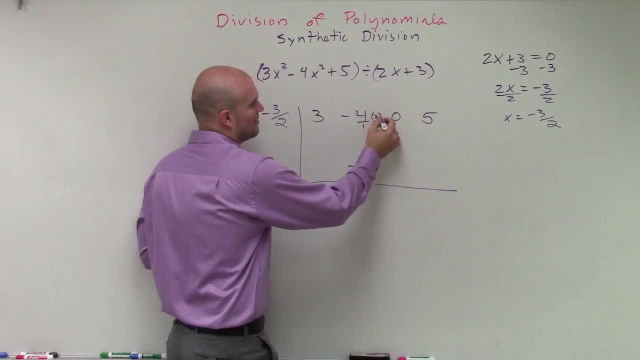 over. so multiply by, convert that to 1,, multiply by 2 over 2.. So therefore we have a negative 8 over 2.. Well, therefore, you can see this is a negative 17 over 2.. Then I'm going to multiply over. 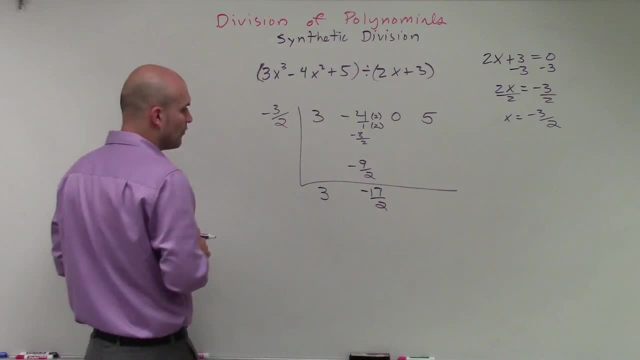 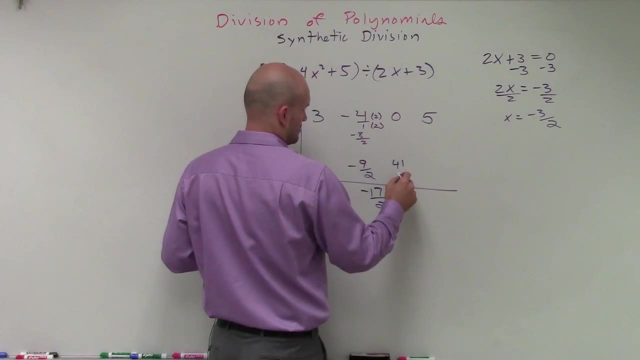 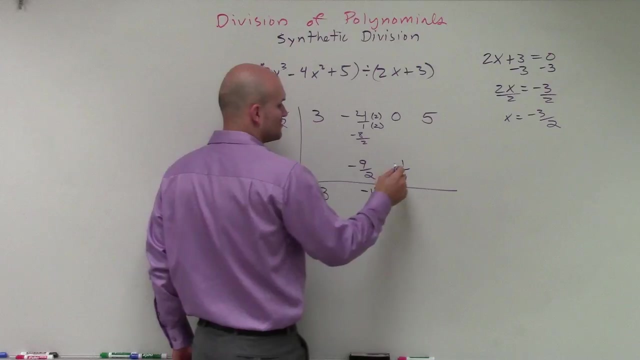 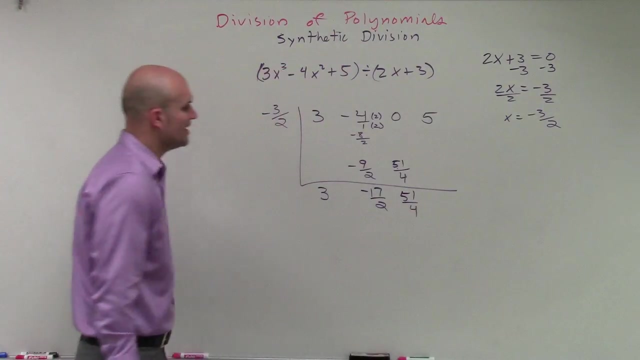 So this would be a 31,. so it would be a positive 41 over 4.. sorry, not 34.. That's already 34, so it's going to be a 51 over 4.. Add those up, Then I need to multiply. 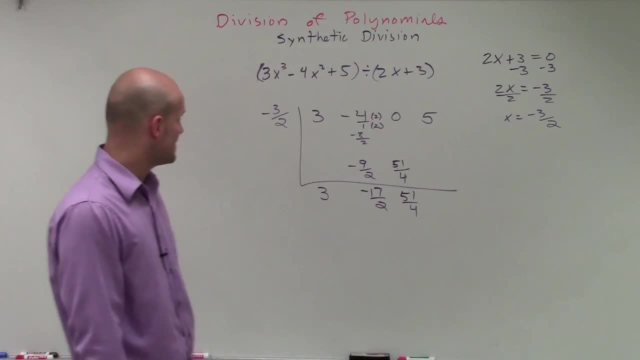 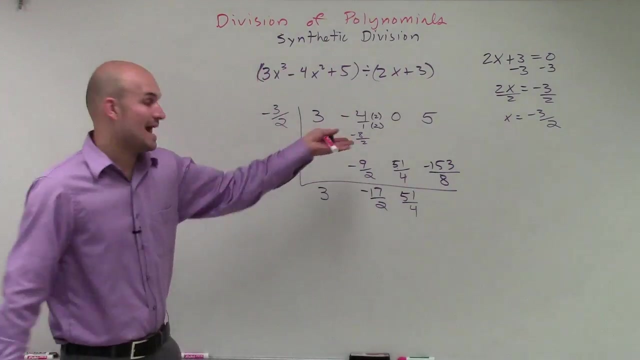 again across. So I have 51 over 4 times negative, 3 over 2. So 51 would be times 2 would be 102, which would be 153, a negative 153 over 8. Then I need to make sure I add: 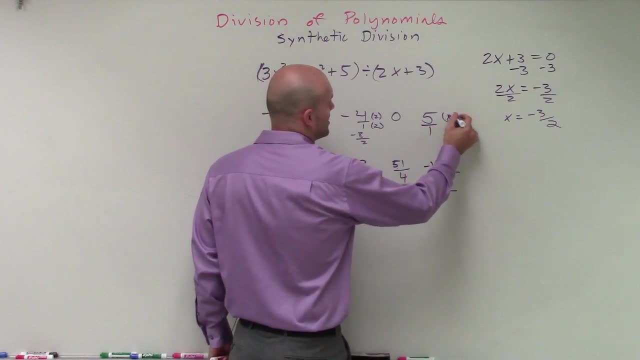 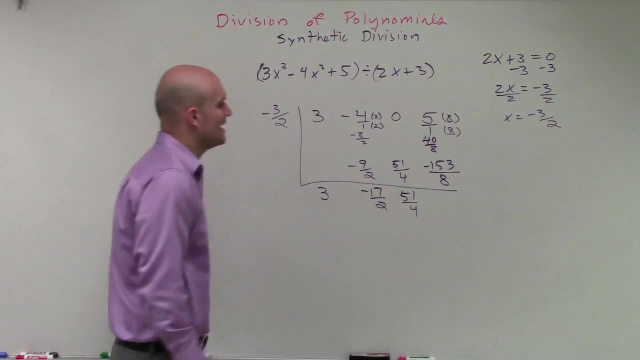 these up together, So this is 5 over 1. to get the same denominator, I'll multiply by 8 over 8. That will give me 40 over 8.. So therefore, then I add these up and you can see that in this case, 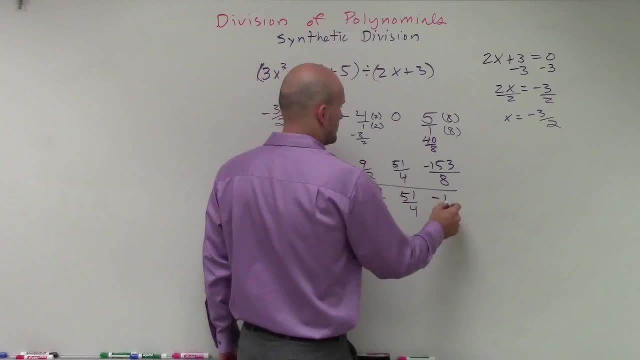 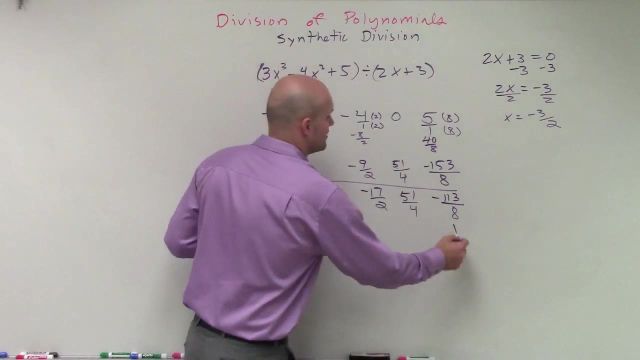 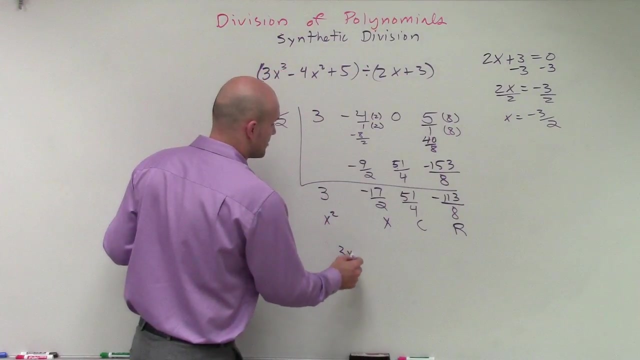 I will have a negative 113 over 8.. So therefore, that's going to be our remainder. Yeah, it's a fraction, but that's okay. Remainder constant, linear Quadratic. So my final solution in this one is going to be a 3, or my final. 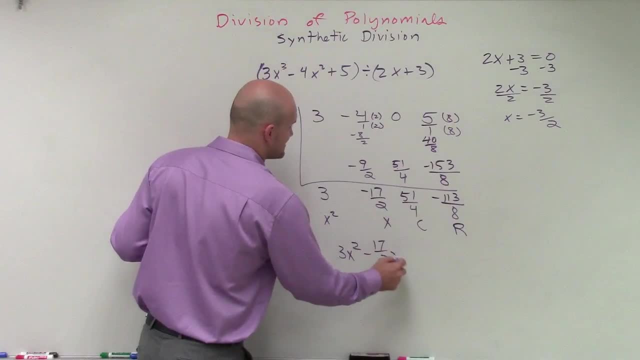 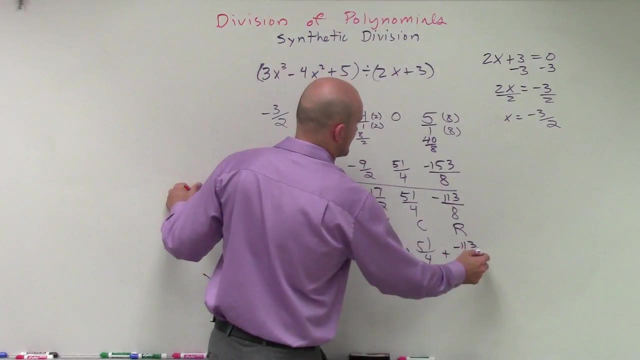 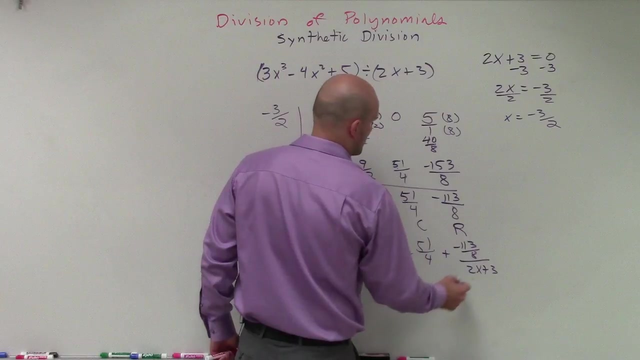 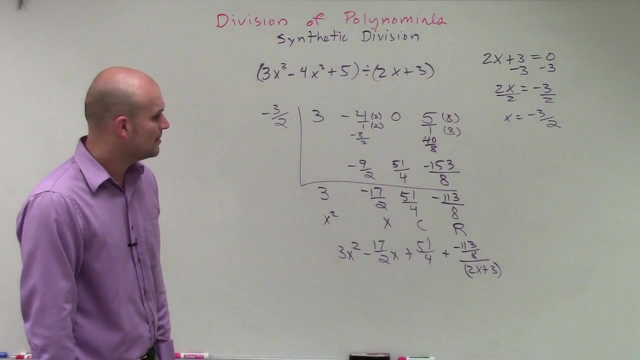 quotient will be 3x squared minus 17, halves x, plus 51 over 4, plus a negative 113 over 8 divided by 2x plus 3.. And then there's a couple different ways. we could probably rewrite that to put that on top, so we could. 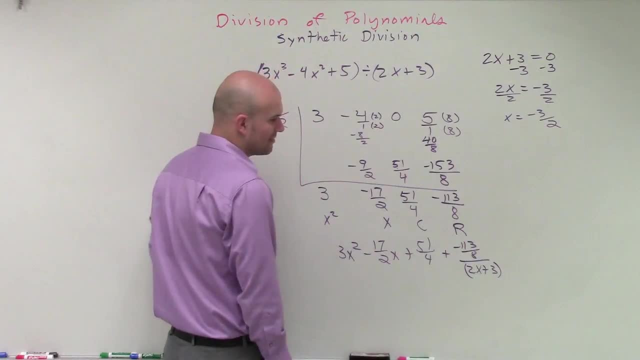 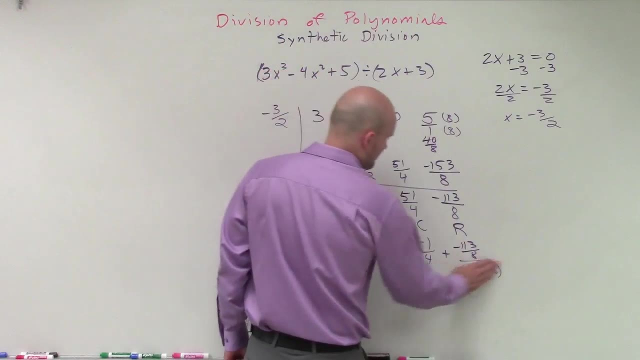 take our divisor and then rewrite that, or multiply this by our reciprocal over here. So really, let's rewrite that, so it's only one fraction times 2x plus 3.. So there you go, ladies and gentlemen. That is how we solve one of those problems. 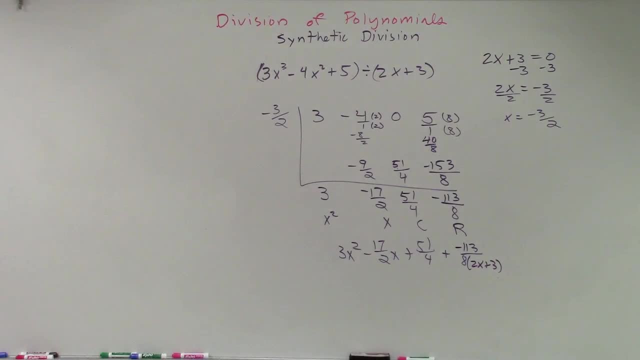 Thanks. Thank you so much for watching. We'll see you next time. Bye, Bye, Bye, Bye, Bye.